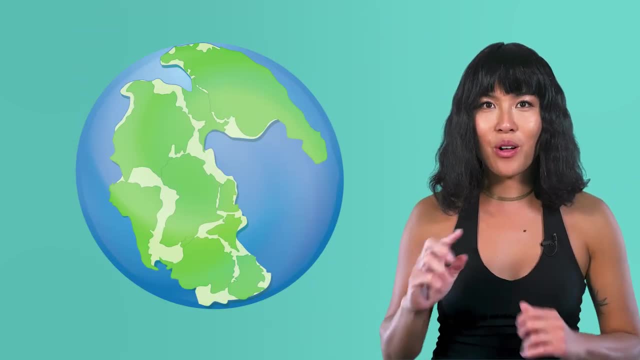 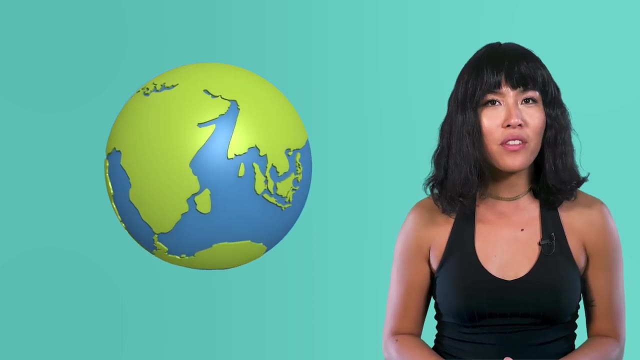 the Earth used to just have one supercontinent, and the Earth's continents were just one supercontinent called Pangea that slowly drifted apart into the seven continents we know today. Alfred called the theory continental drift, or the slow movement of continents across. 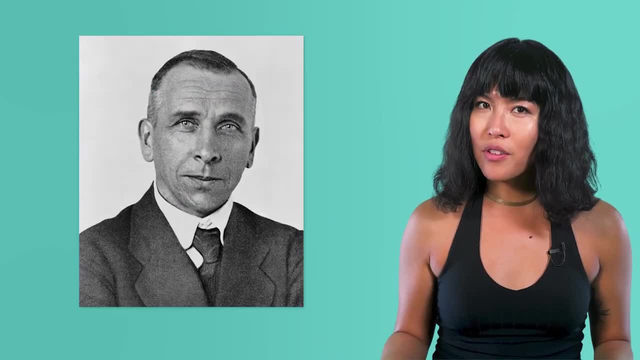 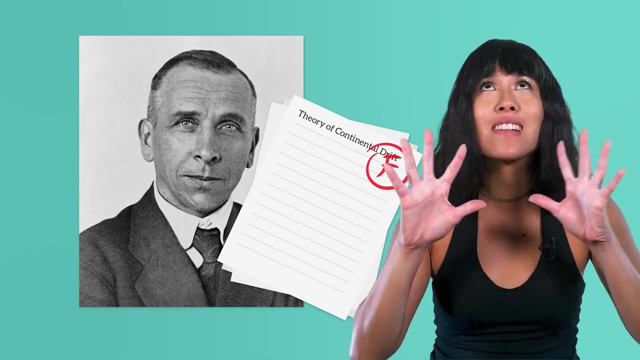 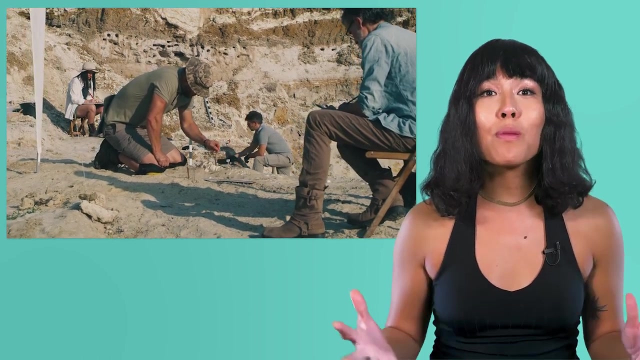 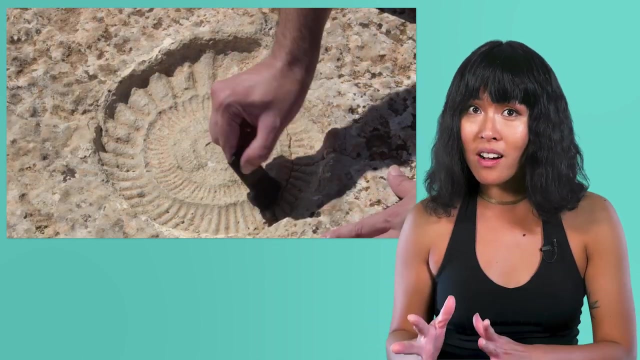 Earth's surface. Unfortunately for Alfred, nobody believed his theory of continental drift. After all, it's pretty hard to imagine entire continents just drifting across the ocean. But decades after Wegener's lifetime, more and more evidence began emerging that supported his theory. Fossils of animals only thought to have lived on one continent were found on the other. 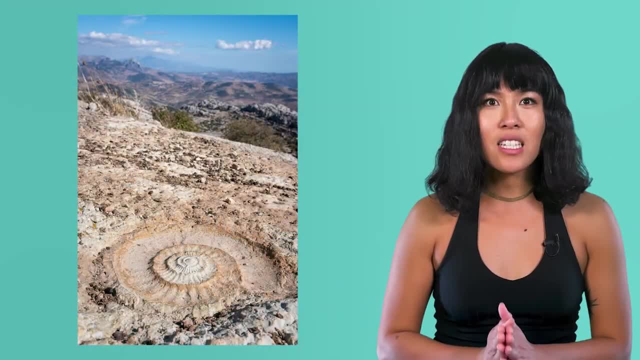 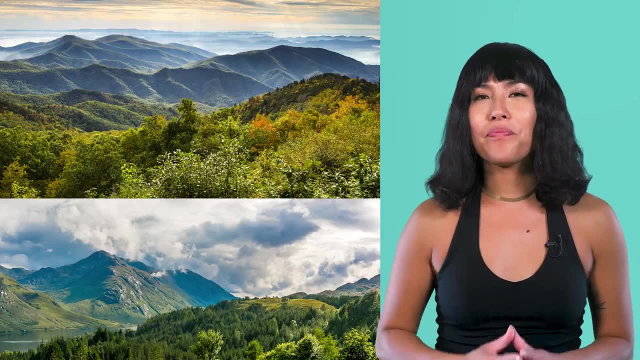 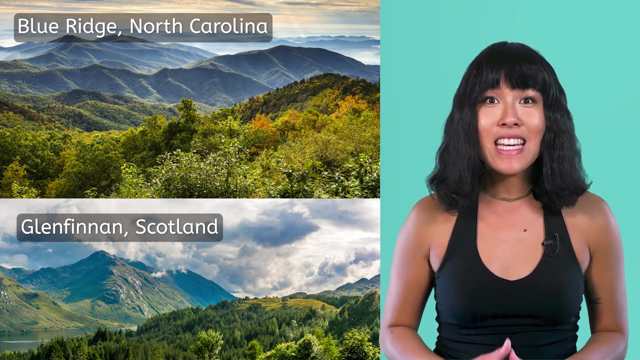 side of the ocean too. Then scientists realized that the rocks the fossils were found in also matched. Here's an example: There are nearly identical mountain ranges made of the same kind and age Age of rocks in Europe and North America. How do you think that happened? 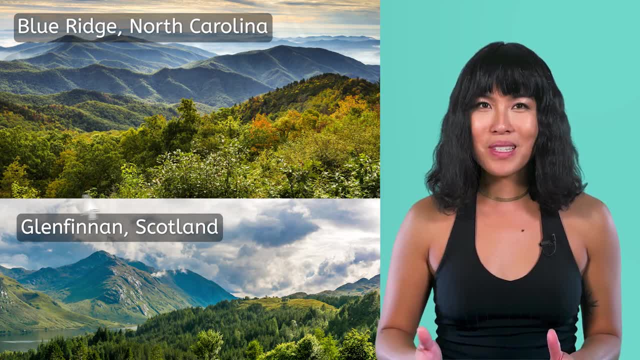 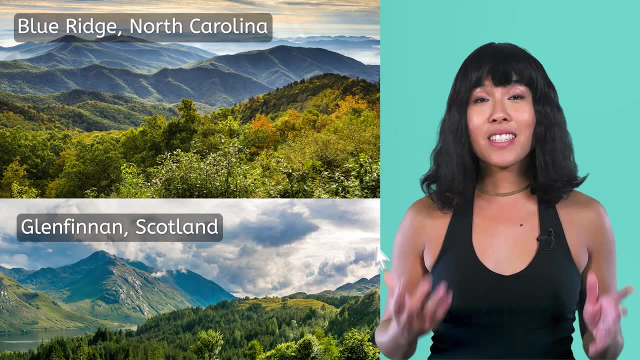 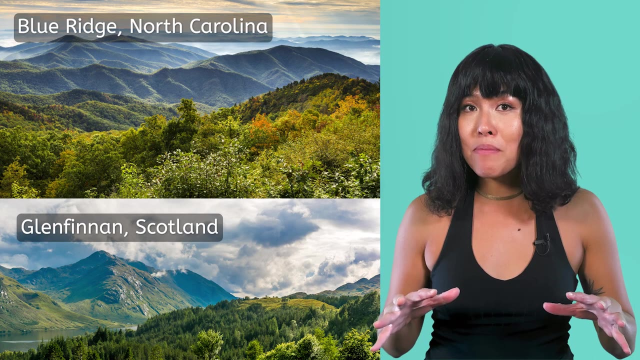 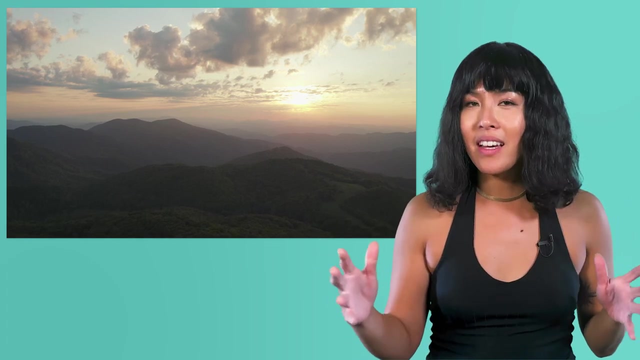 Pause the video here and write down your thoughts in your guided notes. Discoveries like these gave scientists some hard questions to answer. Did these mountains form at the same time in different locations, Or did they form as one mountain range? Continental drift was starting to sound more plausible, But the problem with Wegener's theory. 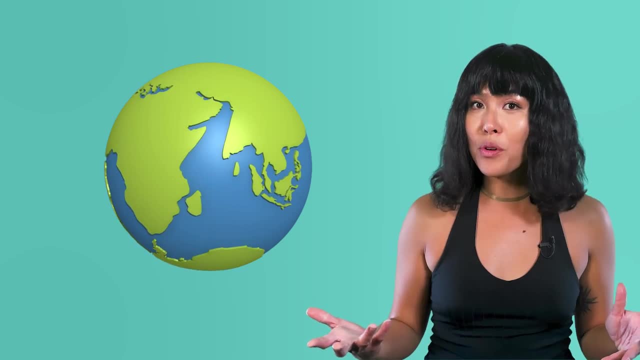 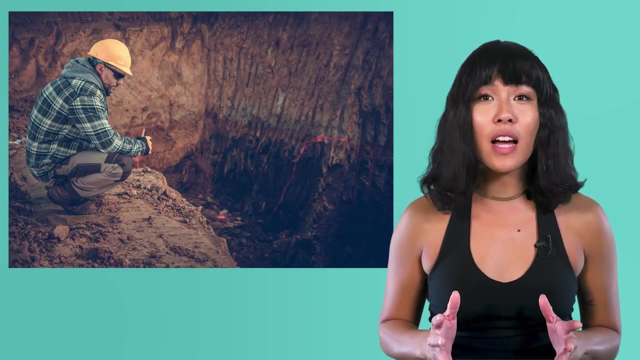 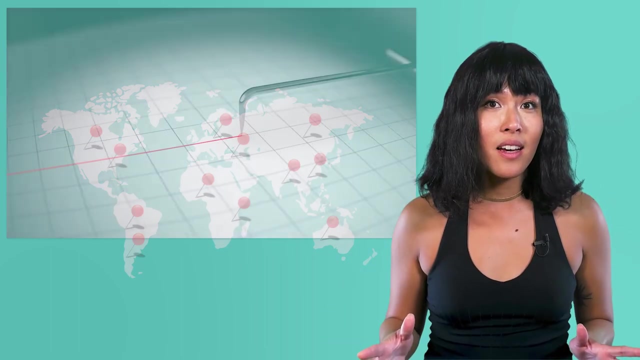 was that it didn't explain how the continents were moving. That's where the theory of plate tectonics comes in. This theory started out with scientists who study earthquakes. They used to think that earthquakes just occurred randomly all across the planet. But as technology got better, 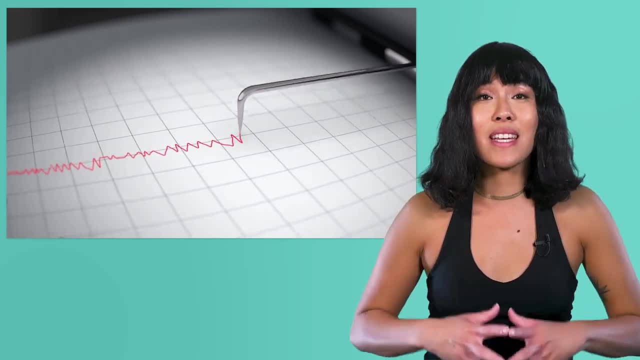 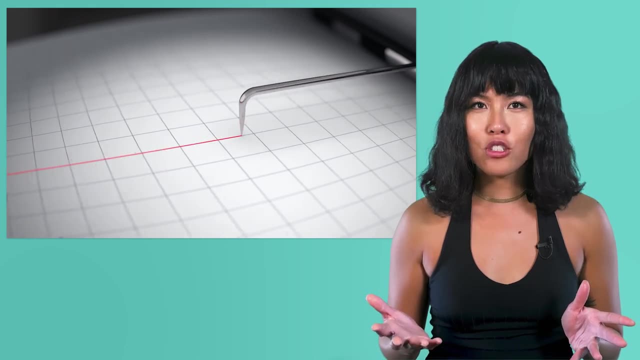 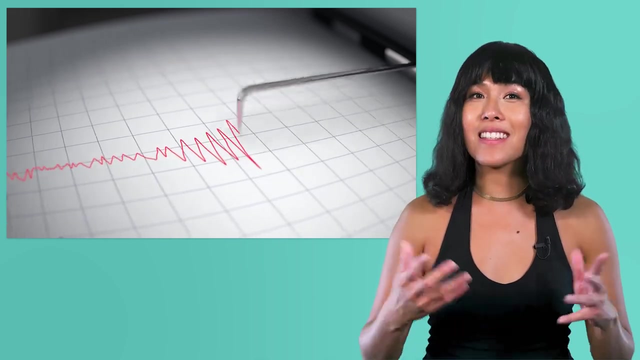 and better. throughout the 1900s, they began to think that earthquakes were just a matter of nom Blick, But in the early 2000s scientists started making tons of new discoveries. A seismograph turned the earth into electric signals and used them to learn more about earthquakes as they 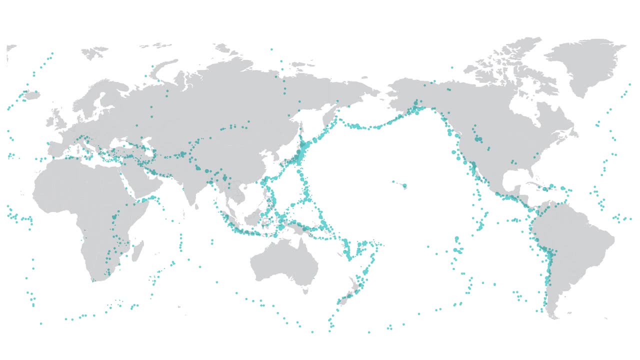 occurred. These events usually happened from different places. Like參Like to Earth Sat on Europeans terminus Doppler. they show them that these events in Earth's crust usually only happened in certain places, And they happened in those places over and over again. 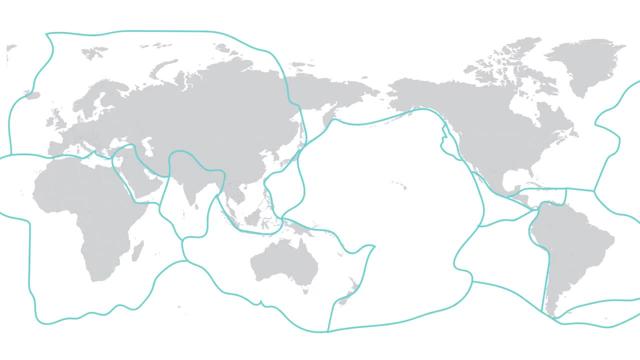 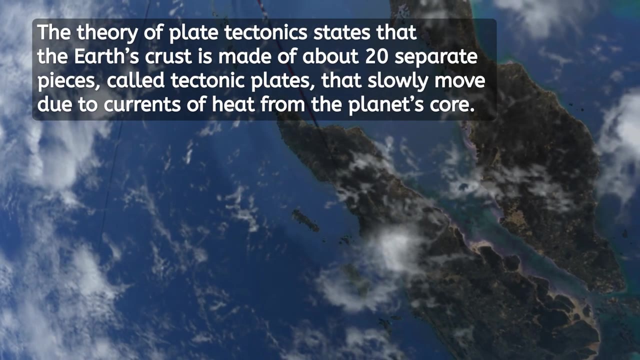 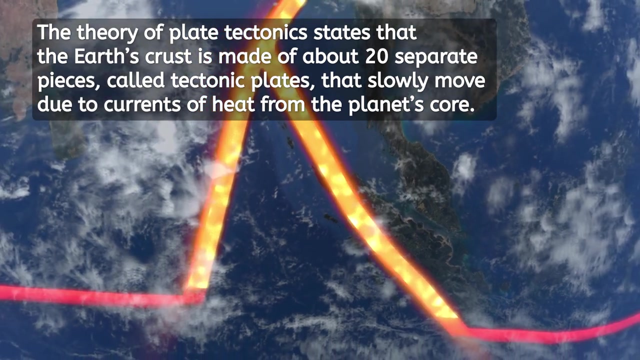 The Earth was formed during the twelfth century and by the time teaser of The Web is full again xu 현. By mapping out the lines along which the earthquakes tended to happen, scientists mapped out divisions in the Earth's crust. The theory of plate tectonics states that the Earth's crust is made of about 20 of these separate pieces called tectonic plates. 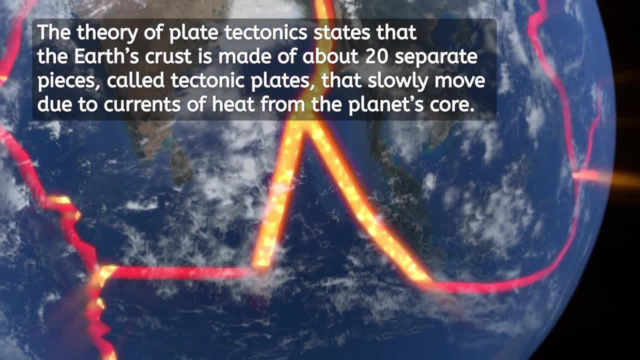 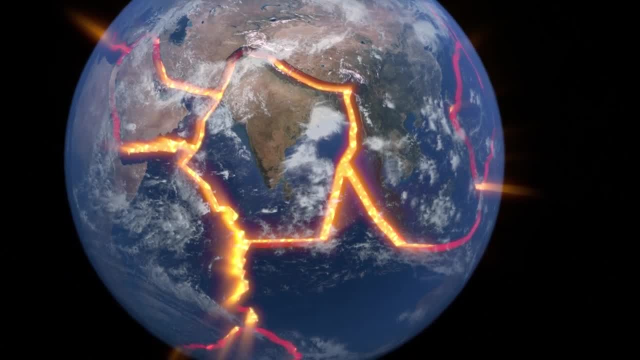 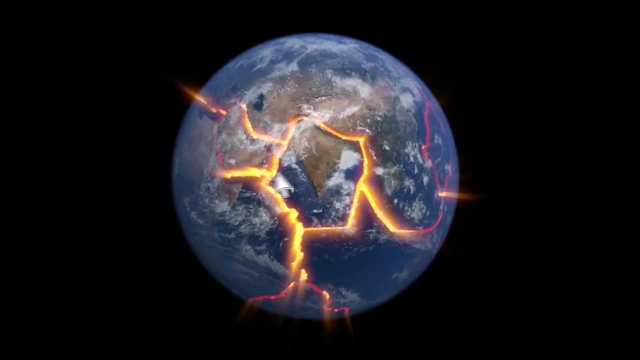 that slowly move over time due to currents of heat from the planet's core. So how do you think the theory of plate tectonics changed the way people thought about the theory of continental drift? Pause the video here and write your thoughts in your guided notes. 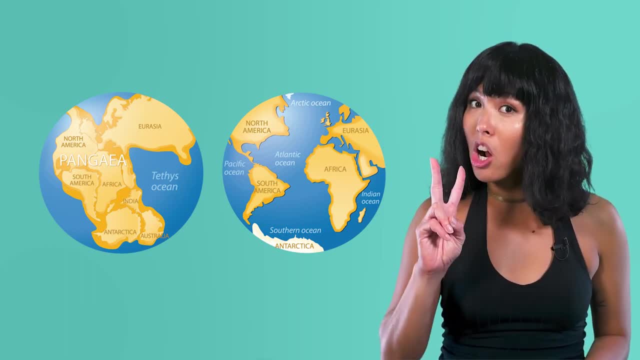 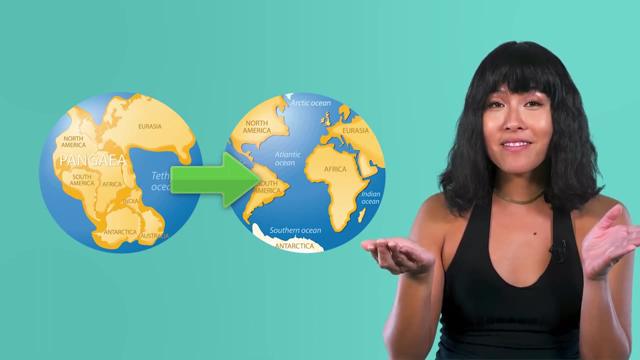 Scientists started to see how these two theories are closely related. Basically, plate tectonics are the cause and continental drift is the effect. So how do you think the theory of plate tectonics changed the way people thought about the theory of continental drift? 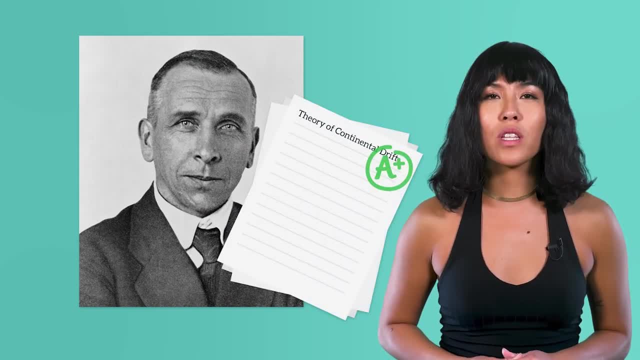 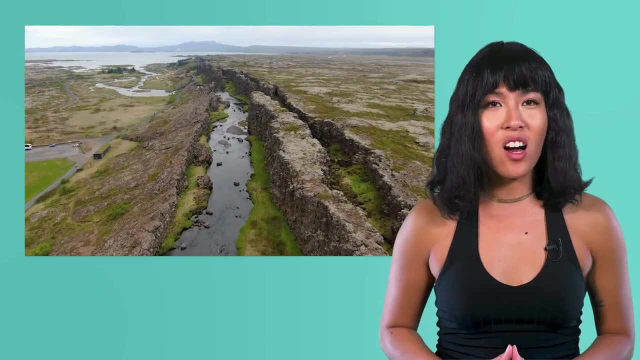 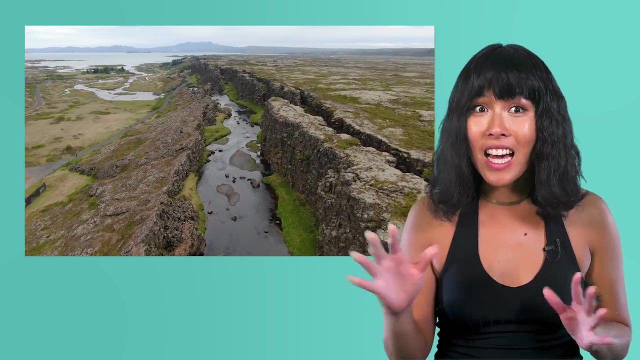 Alfred Wegener's theory started to make a lot more sense once we had an idea of how it could be possible for a continent to move. There are places along the edges of tectonic plates where we can actually see how the Earth's surface changes as a result of this movement. 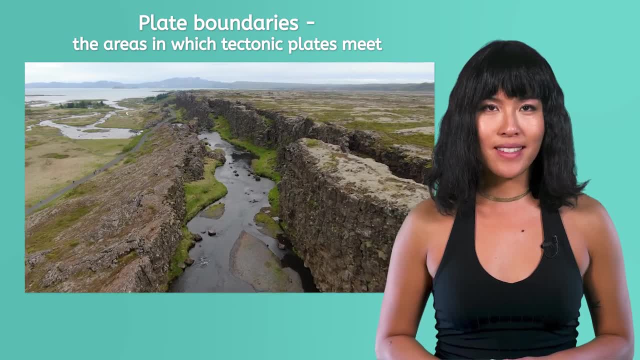 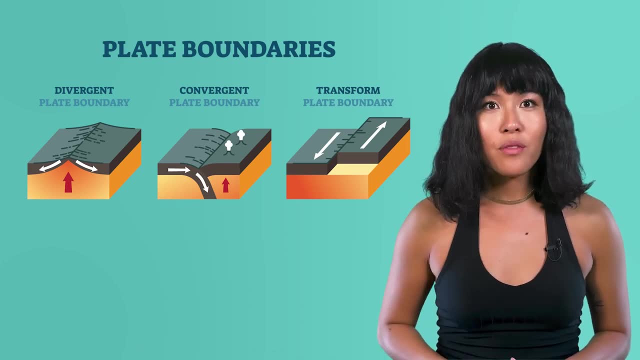 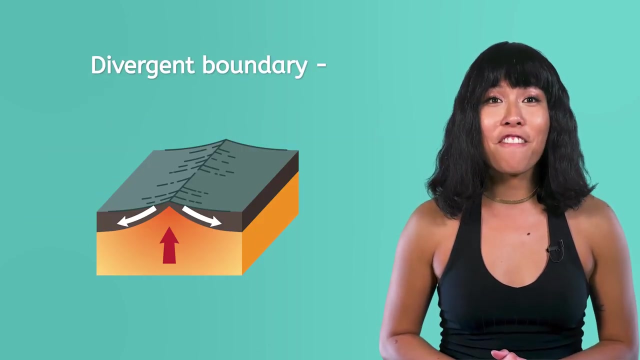 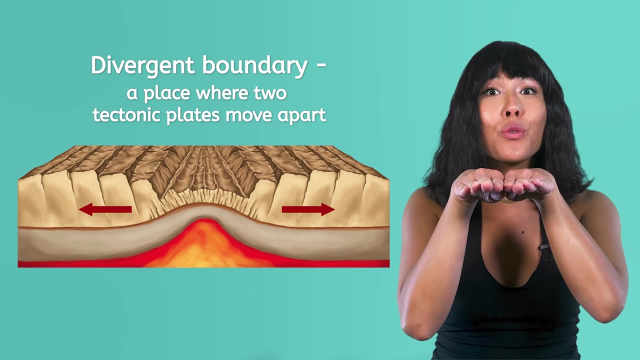 These edges are called plate boundaries, the area in which tectonic plates meet. There are three different kinds of plate boundaries, One for each of the three different ways they can move. The first is called a divergent boundary. Diverge is another word for separate, so a divergent boundary is a place where two tectonic plates are moving apart from each other. 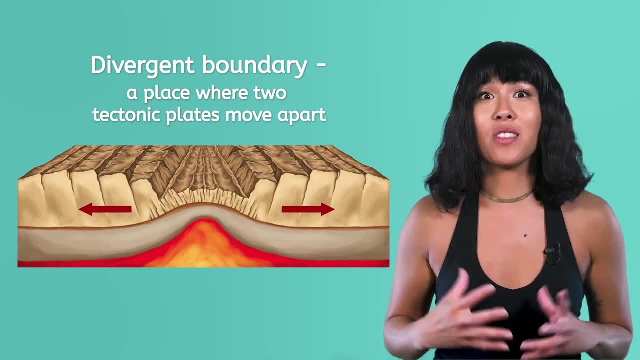 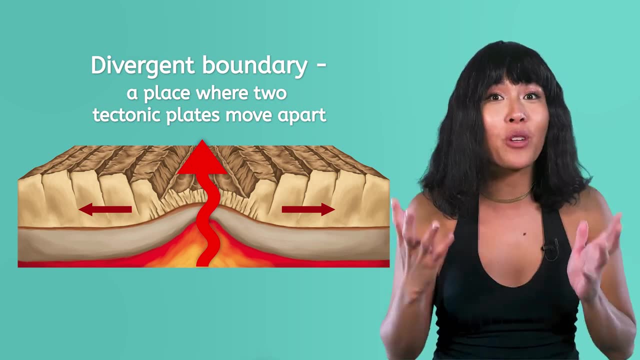 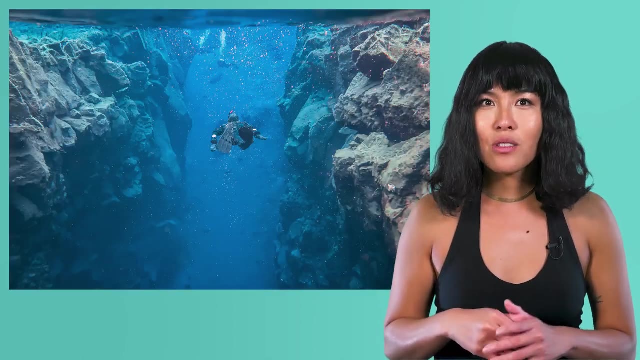 As they pull apart. the movement often causes earthquakes and creates areas where molten rock from the Earth's mantle can rise to the surface in volcanoes. Over time, water rushes in to fill the new gap in Earth's crust. In fact, there is a place in Iceland where you can swim between two tectonic plates in a divergent boundary. 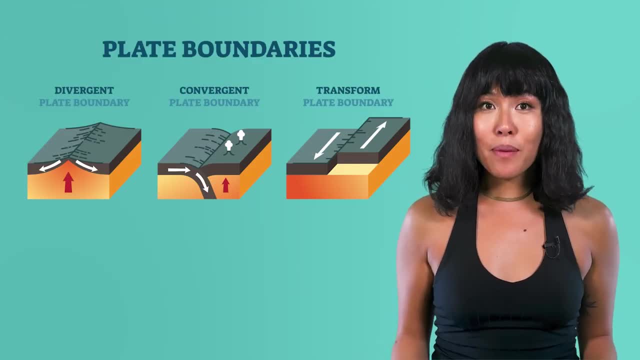 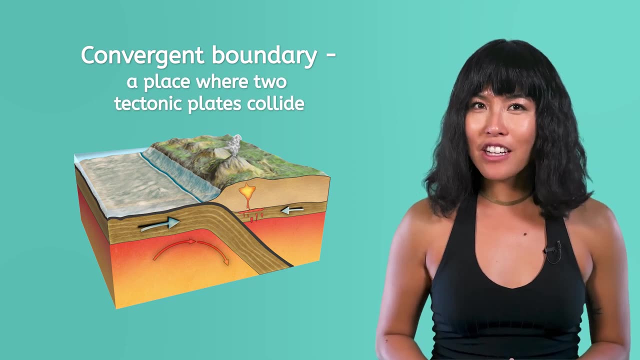 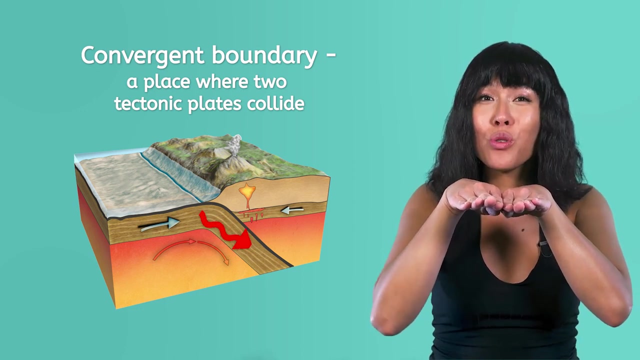 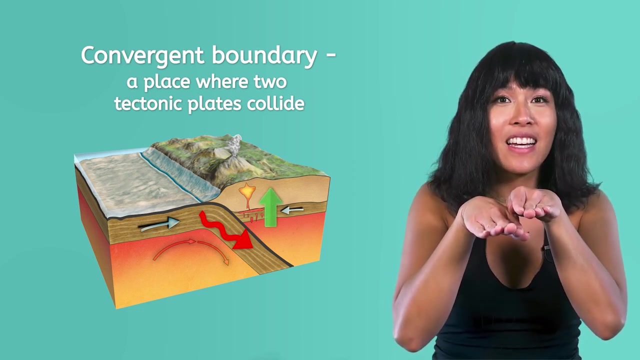 Pretty amazing, huh. The next kind of plate boundary is a convergent boundary. Converge means to come together, So you guessed it. This kind of boundary means that two plates are colliding. When this happens, the denser plate will usually be pushed down underneath the lighter plate and melt, leading to volcanic activity. 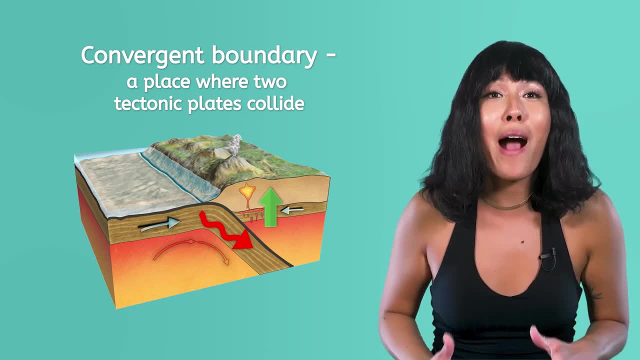 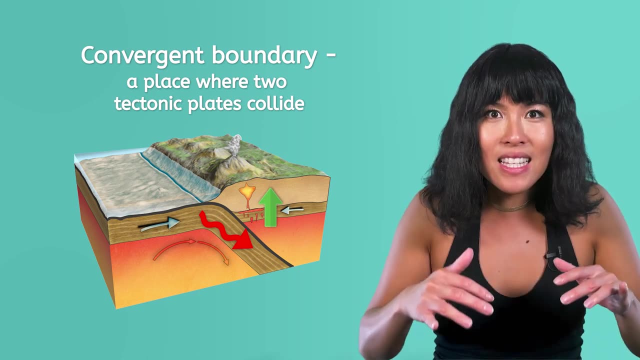 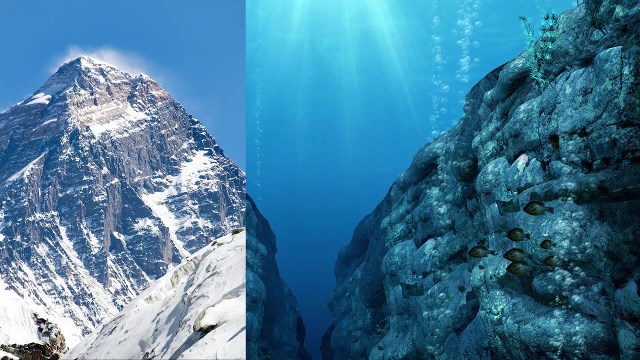 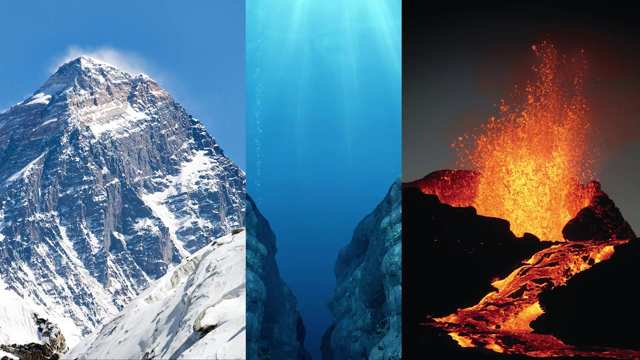 This lifts the lighter plate upwards, resulting in powerful earthquakes, but also creating huge mountain ranges and sometimes even bending the sea floor to create deep trenches. The deepest trench in the oceans, the highest mountain on Earth's surface and the most active volcano in the world were all created by convergent boundaries. 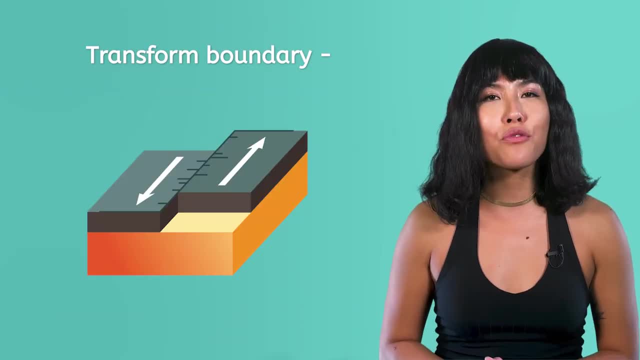 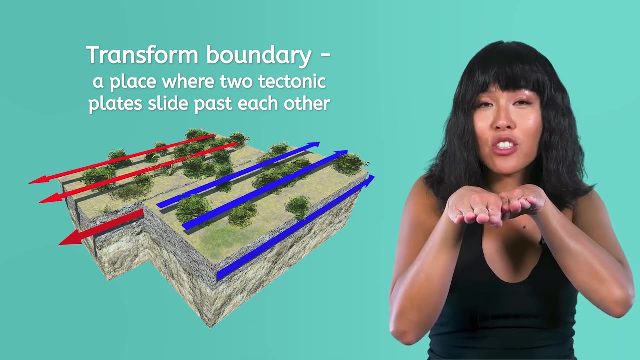 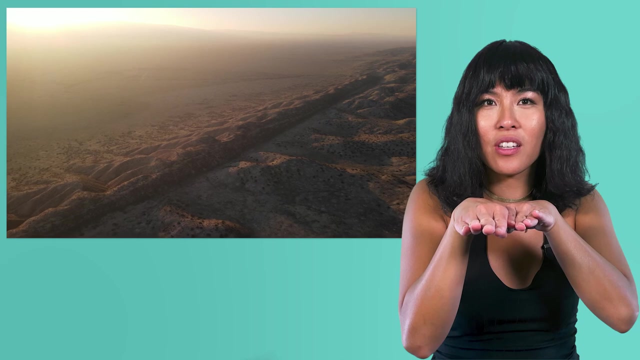 And the last kind of plate is called a transform boundary. This happens when two plates are sliding past each other. These boundaries don't create mountains or melt down tectonic plates, but the constant grinding past each other does create a lot of earthquakes. 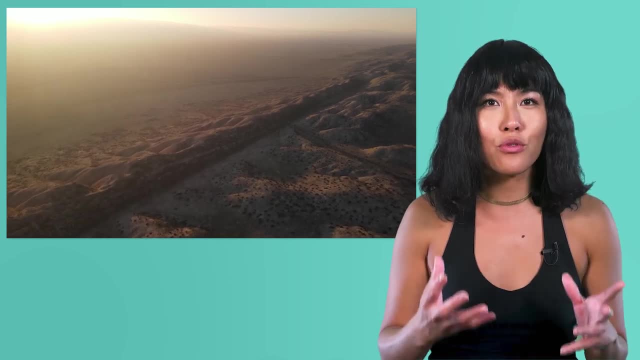 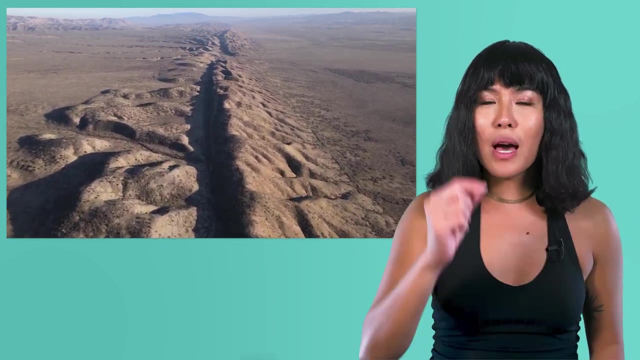 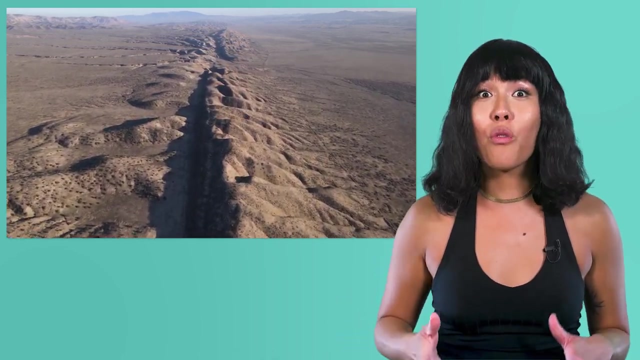 The San Andreas Fault Zone in California is a transform boundary and it is one of the fastest changing plate boundaries in the world. It moves about two inches every year. It might not sound all that fast, but over time it's enough to move continents. 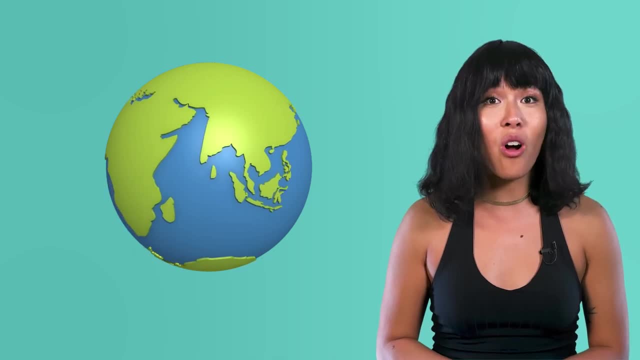 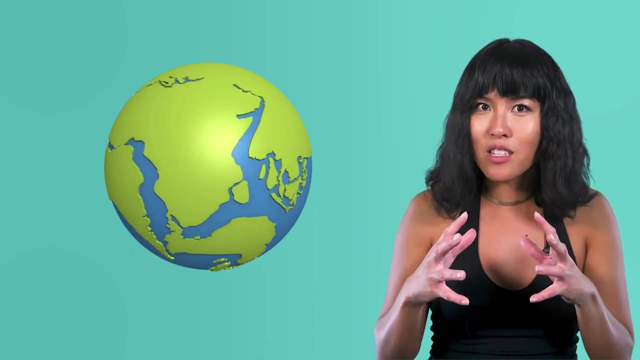 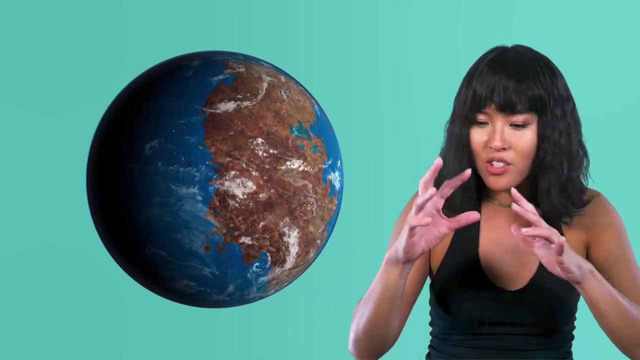 And yes, that does mean that the continents are all still in motion today. Scientists think that in the distant future they'll all merge together again to form another huge supercontinent, But they aren't exactly sure what it will look like or where each continent will end up. 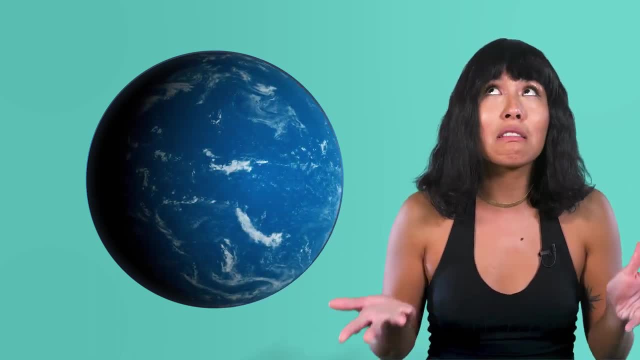 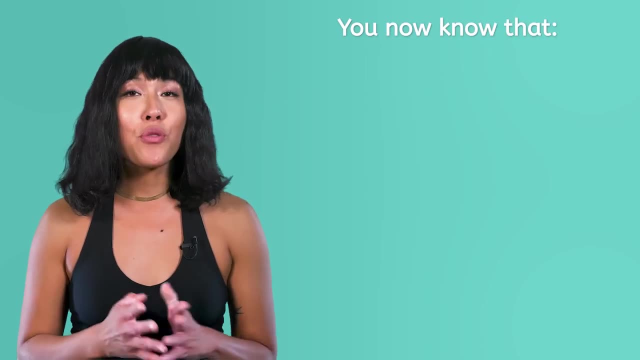 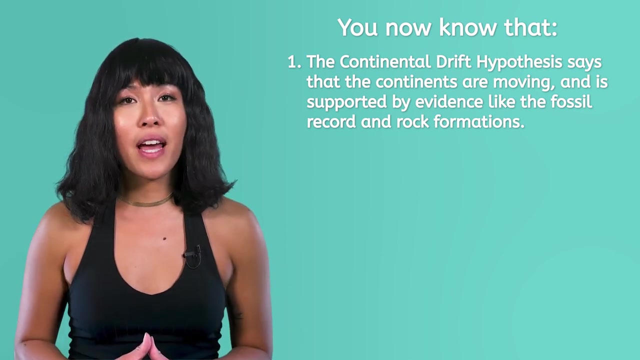 But don't worry, we'll only need to wait another hundred million years or so to find out. So let's recap what we learned today. You now know that the Continental Drift Hypothesis says that the continents are moving and is supported by evidence like 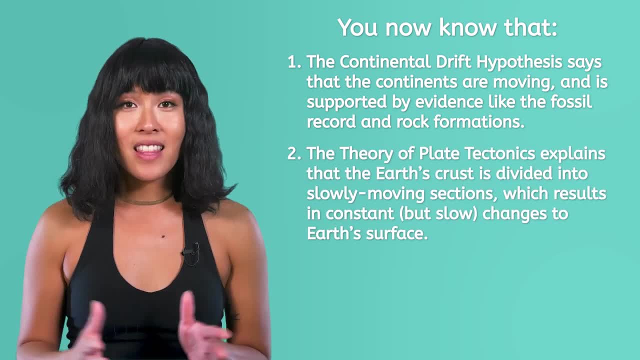 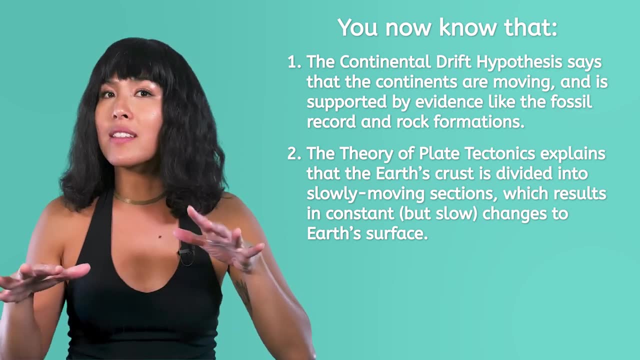 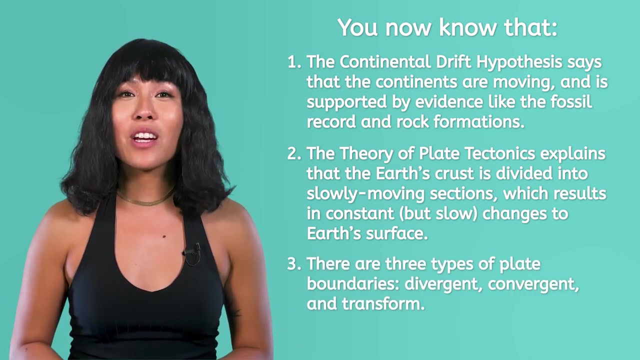 the fossil record and rock formations. The theory of plate tectonics explains that the Earth's crust is divided into slowly moving sections, which results in constant but slow changes to Earth's surface, And there are three types of plate boundaries. 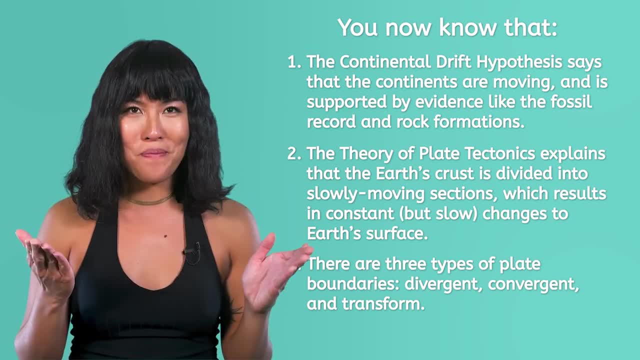 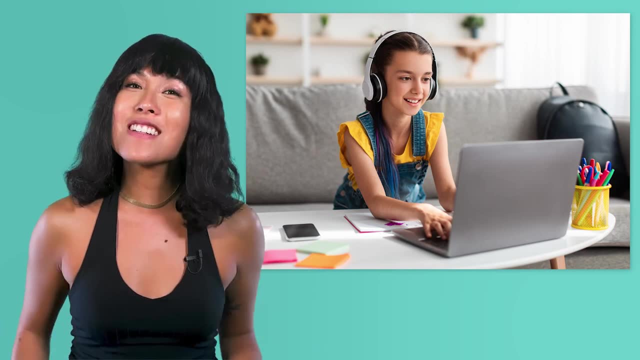 divergent, convergent and transform. Now that we've solved this puzzle, be sure to check out the games and extension activities to help you get ready for our next lesson, when we'll learn even more about how plate tectonics shape the Earth. 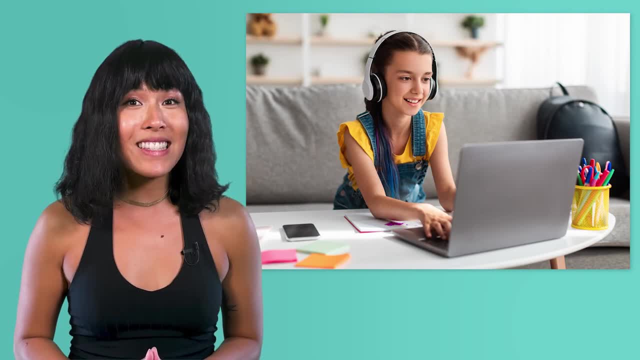 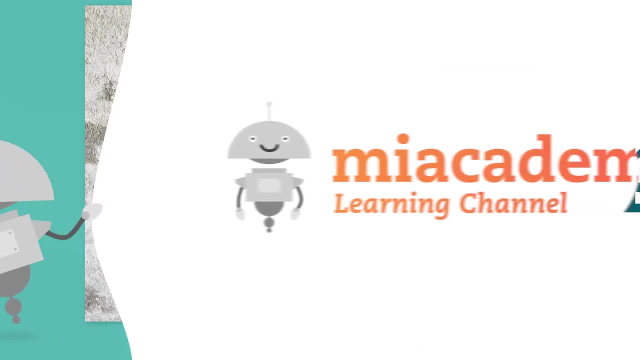 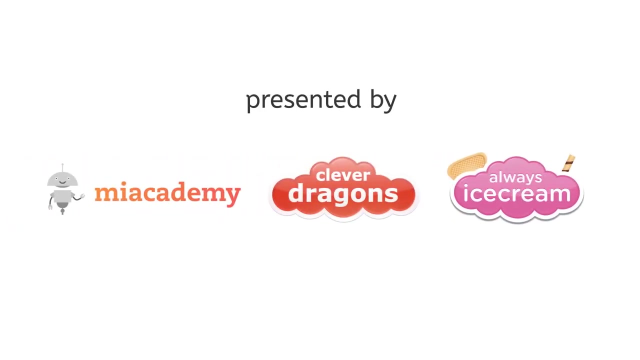 In the meantime, remember, in Earth science as in life, you rock. See you next time. Subtitles by the Amaraorg community. 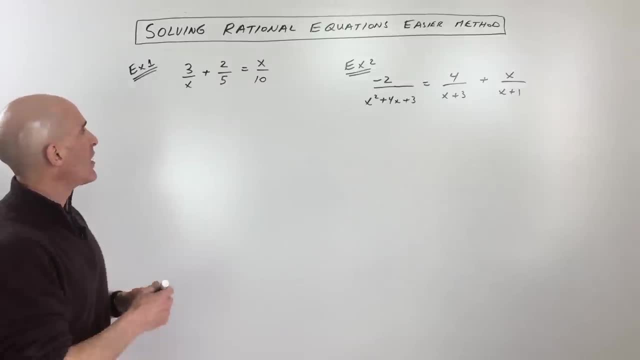 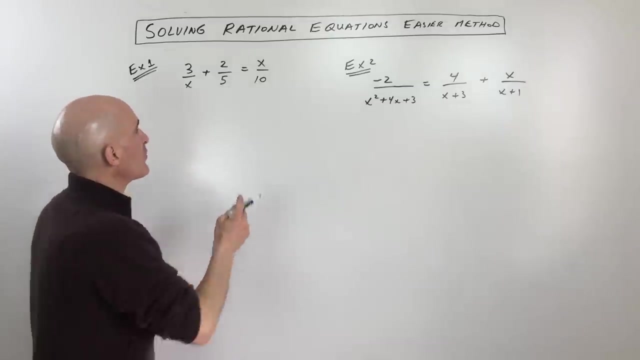 Normally, when they teach this technique in algebra classes is what they'll do is they'll say: we'll find the common denominator and then multiply through by that common denominator to clear the denominators. But oftentimes students get a little bit confused by that, and so what I'm going to show you here is: let's just see if we can get all the denominators to be the same. Okay, so here you can see: this has an x, this has a 5, and this has a 10.. Okay, we want all these denominators to be the same. So if we can make all these denominators, 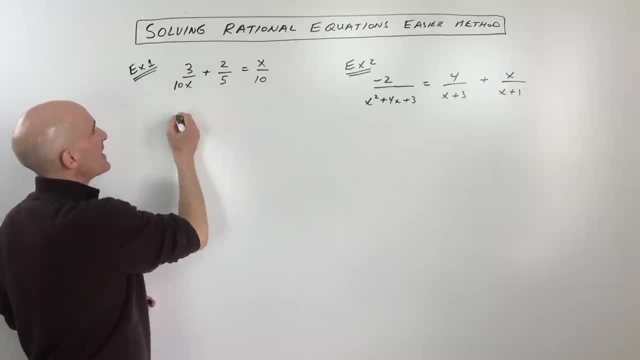 10x. See, because this one has an x, it's missing a 10 right. So if I multiply that by 10, I have to make sure I do it to the top and the bottom, So you can see I have 10 times 3 over. 10x now Over. 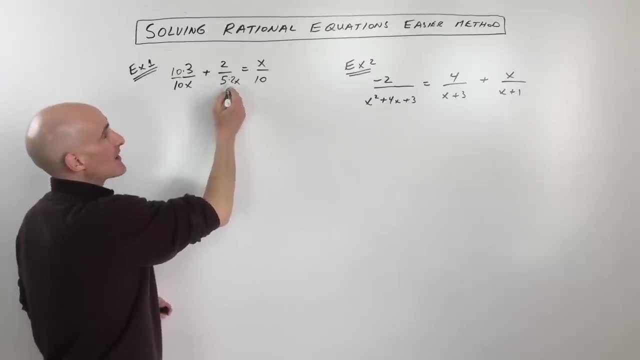 here I really need a 2 and an x to make this 10x. Okay, so I'm going to multiply the top and bottom by 2x. and then here I'm just missing an x, so I'm going to multiply the top and bottom by x. Okay, 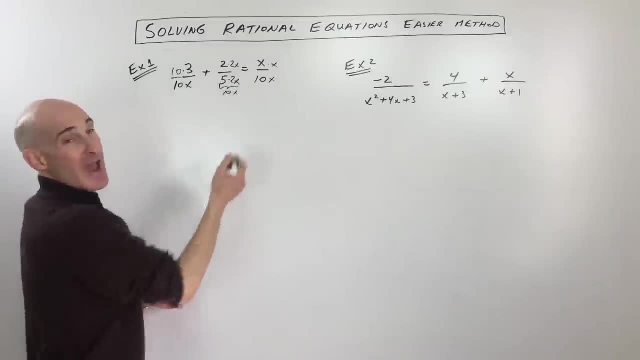 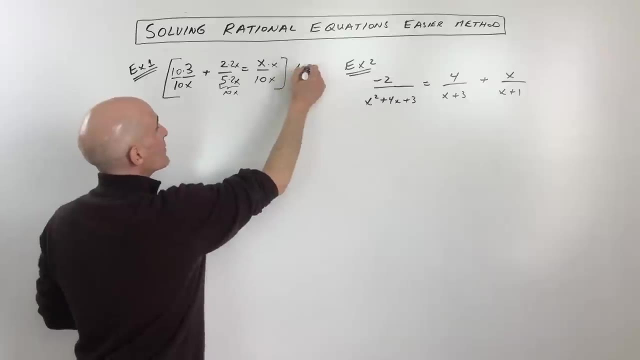 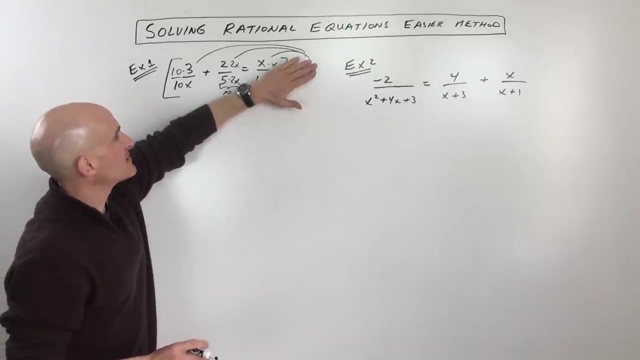 so now you can see that all the denominators are 10x. So now what I would do is I would say: all right, I'm going to multiply everything by this denominator, 10x. So when you do that, when you distribute it, okay, what happens is when you multiply the 10x and the 10x, those are going to 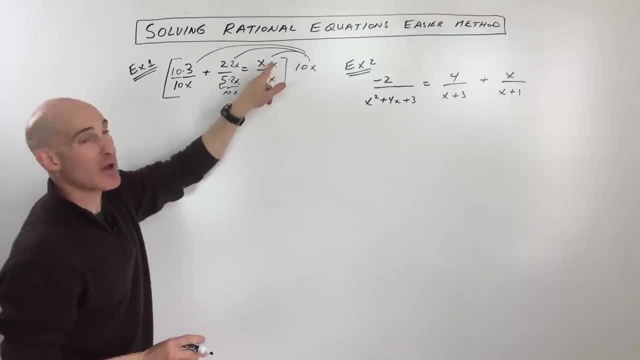 cancel. So what it does is it clears the denominators. You don't want to actually multiply the numerators by 10x, You just want to realize that, since these all have the same denominator, if you were to multiply through by that common denominator, you're just going to be.